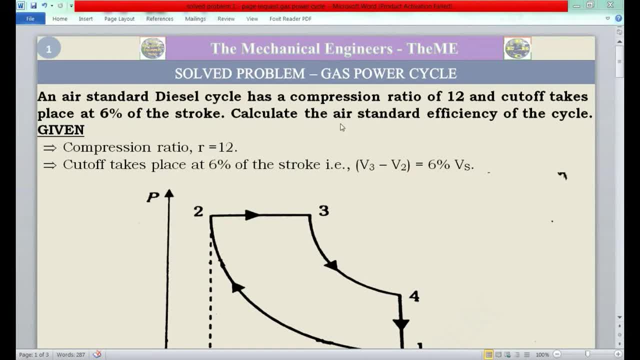 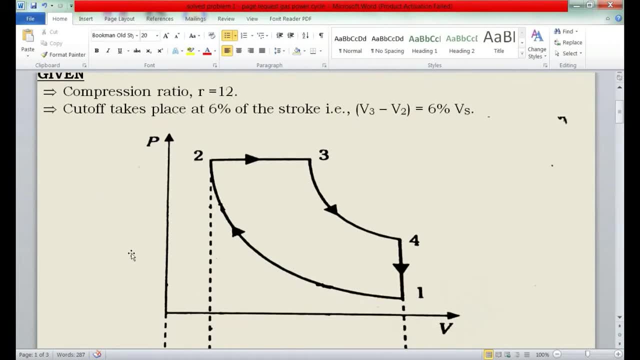 cycle. So in this question we have to find the air standard efficiency of the cycle. First we will look into the PV diagram of diesel cycle. So this is the PV diagram, That is pressure volume diagram. So in this pressure volume diagram the pressure values, 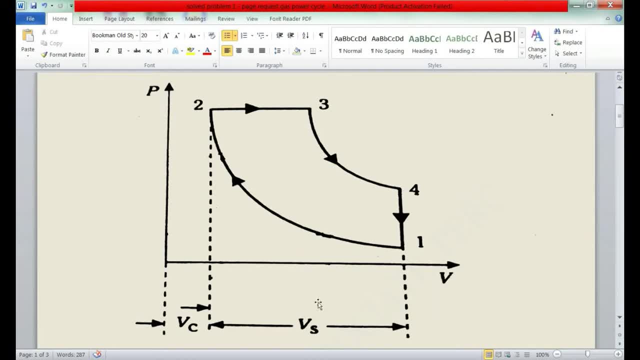 are plotted along y-axis and volume values are plotted along x-axis. This, 1,, 2, 3, 4 are the pressure and volume values at different state. To make it more simple, this 1 is nothing but the pressure and volume value at state 1,, which is P1, V1.. This 2 is nothing but. 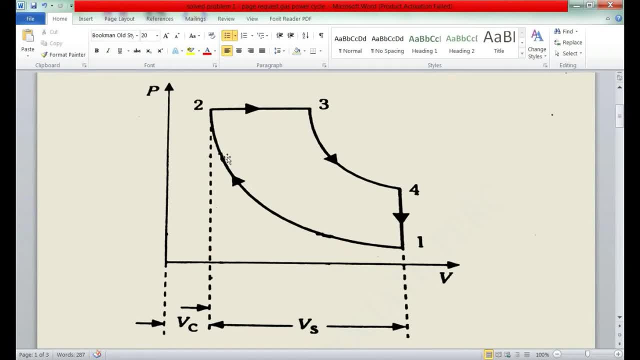 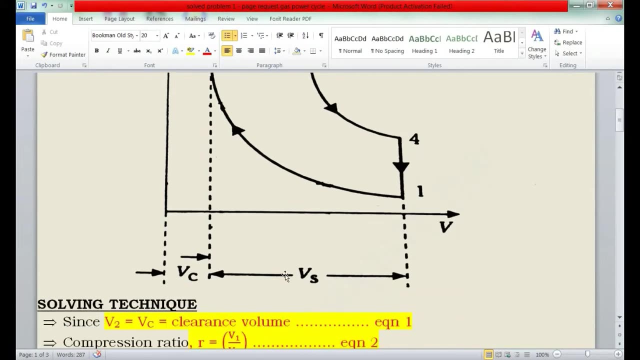 the pressure and volume value at state 2,, which is P2, V2.. This 3 is nothing but pressure and volume value at state 3,, which is P3, V3.. And 4 is nothing but pressure and volume value at state 4,, which is P4, V4.. This Vs is nothing but stroke volume. The definition. 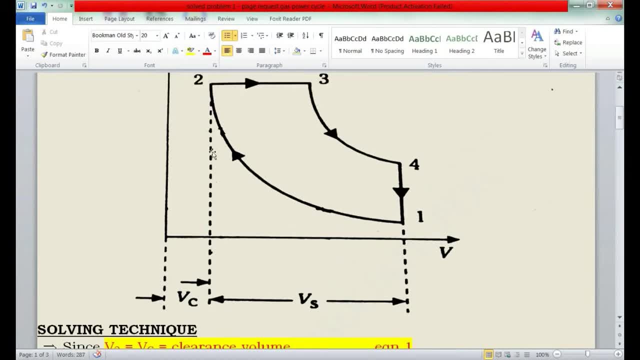 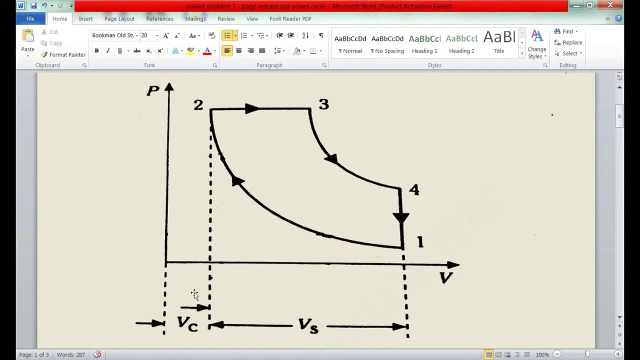 is the volume occupied between V1 and V2.. So the formula is: Vs is equal to V1 minus V2.. And this Vc is nothing but clearance volume, which is also V2.. So this volume is nothing but V2, which can be called as clearance volume, or you can simply: 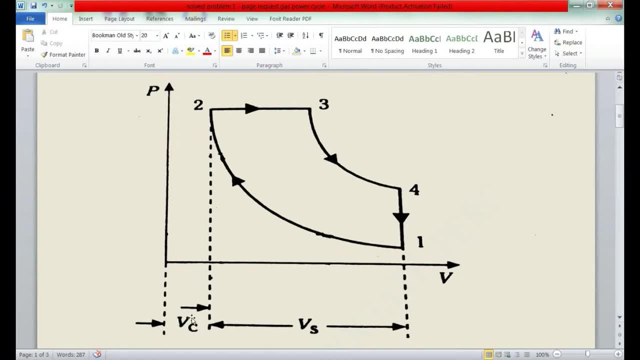 say it as V2.. So the condition is Vc is equal to V2.. In diesel cycle there are four different process. The first one is process 1 to 2, which is reversible adiabatic compression process. So in this process there will be 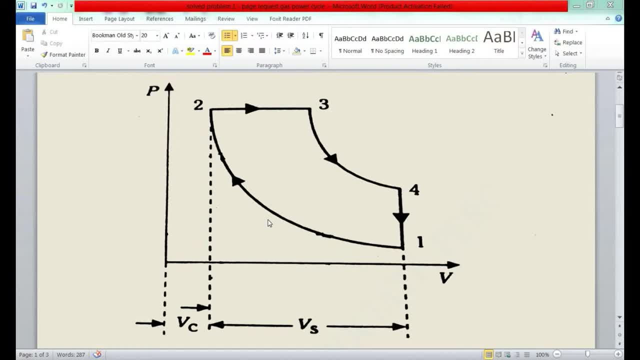 no heat addition or heat rejection. Pressure and temperature will be increased. Volume will be decreased. Next process is process 2 to 3. And this process is a constant pressure process, So P2 is equal to P3. And in this process, volume will be increased and heat. 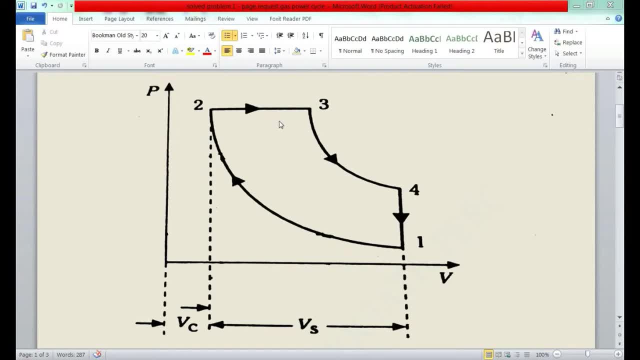 addition takes place, So that the temperature will also be increased and cut off takes place. So these are the condition happens during this process. So next is process 3 to 4, reversible adiabatic expansion process. So in this process there will be no heat addition or 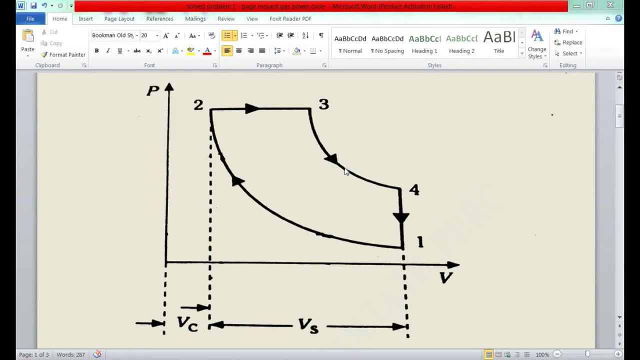 heat rejection. The pressure and temperature will be decreased and the volume will be increased. So next is process 4 to 1, which is a constant volume process. Therefore, V4 will be equal to V1.. The pressure will be decreased and the temperature will be decreased because heat. 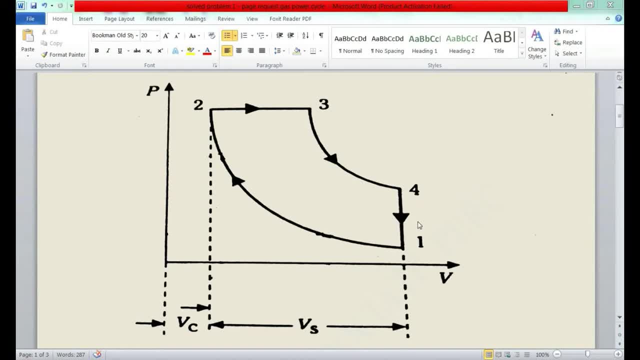 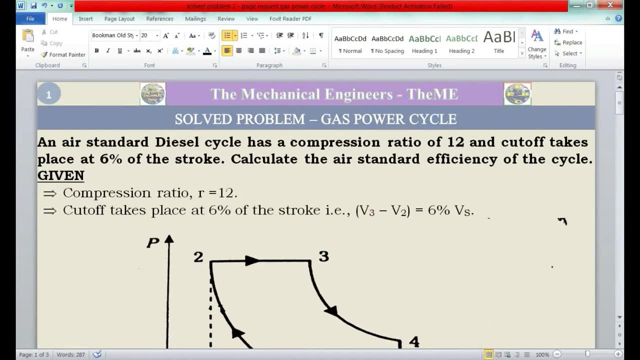 rejection takes place during this process. Now we will list out the given conditions from the question. So the first condition is an air standard diesel cycle has a compression ratio of 12,, which is the compression ratio of this diesel cycle is 12.. So R is equal to 12, where R is the. 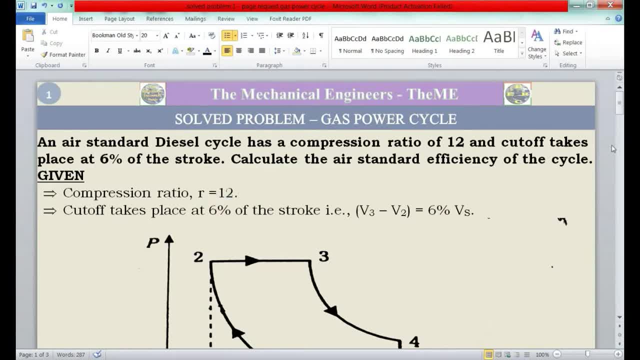 compression ratio. The next condition is: cutoff takes place at 6% of the stroke. Here cutoff is V3 minus V2.. I repeat, cutoff is V3 minus V2 and 6% of the stroke is 6% of stroke volume. 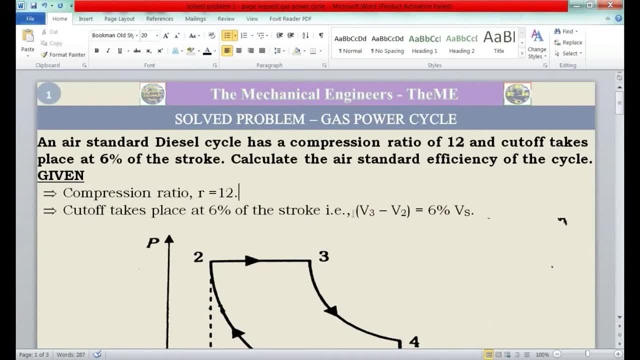 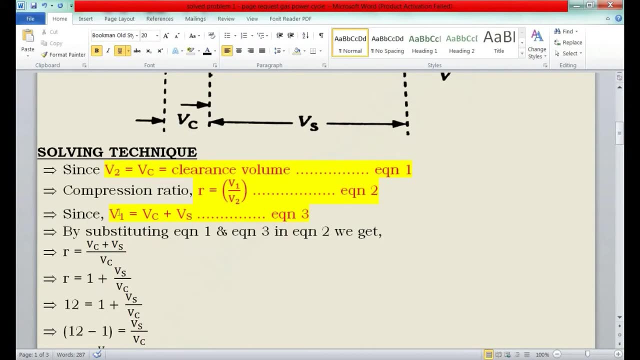 So 6% of Vs. So the equation will be: V3 minus V2 is equal to 6% of Vs. This is the second and final condition. Now we will look into the solving technique. So we know that V2 is equal to Vc. 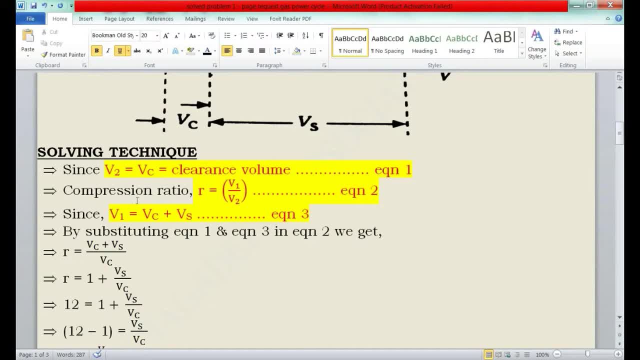 which is clearance volume. Consider this one as equation 1.. Next is compression ratio, and the formula for compression ratio is: R is equal to V1 by V2, that is volume at state 1 divided by volume at state 2.. So this is the compression ratio. So this is the compression ratio. So 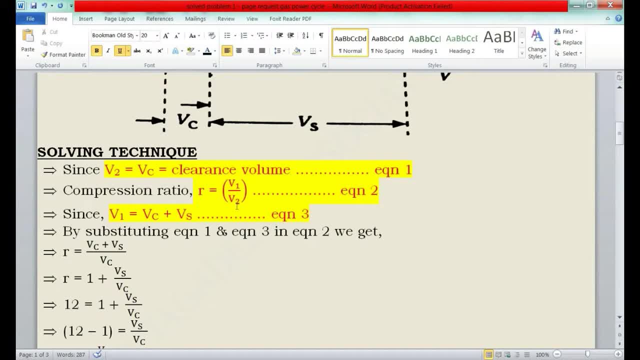 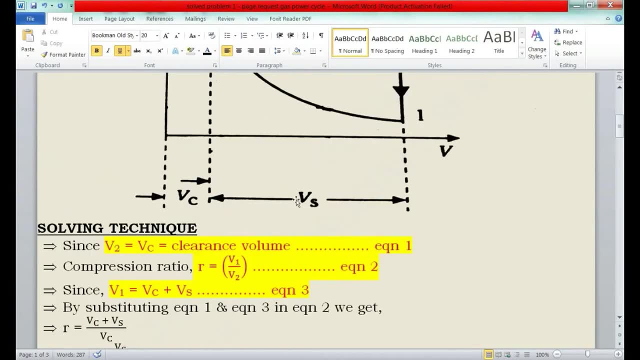 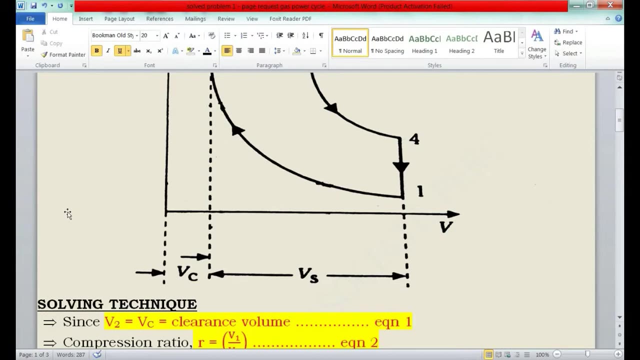 the compression ratio is: R is equal to V2, or volume before compression divided by volume after compression. Consider this one as equation 2.. Next is: V1 is equal to Vc plus Vs. So you can see here in this pV diagram, V1 is nothing but Vs plus Vc. So V1 is equal to Vc plus Vs. 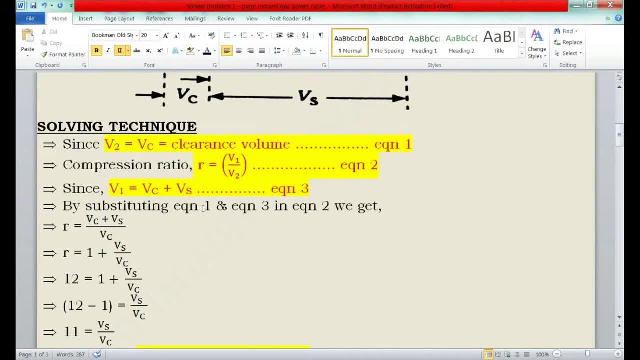 Consider this one as equation 3.. Now substitute equation 1 and equation 3 in equation 2.. okay, Substitute these two equations in equation 2.. So V1 will be replaced by Vc plus Vs, and V2 will be replaced by Vc. okay, So therefore, this equation 2 will be rewritten, as R is equal to Vc. 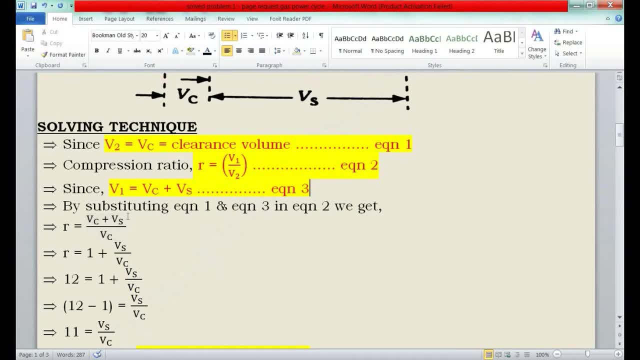 plus Vs by Vc. okay, And this equation will be further simplified, as I mean further modified, as R is equal to 1 plus Vs by Vc, because Vc by Vc is 1 and plus Vs by Vc. okay, We know that R is. 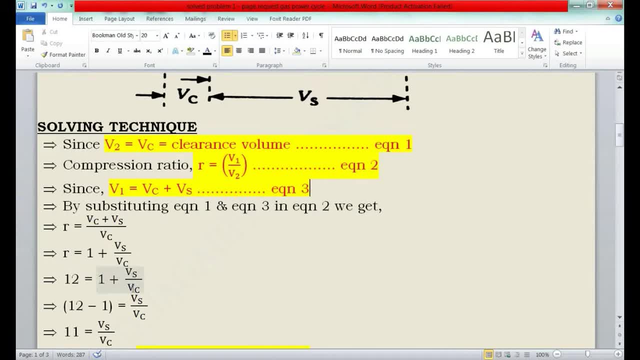 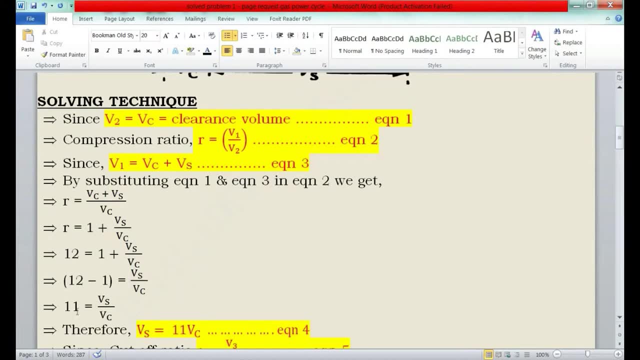 12.. Therefore 12 is equal to 1 plus Vs by Vc. Now move this 1 to the LHS. 12 minus 1 will be equal to Vs by Vc. Therefore 12 minus 1 is 11.. So 11 is equal to Vs by Vc. Now bring this Vc. 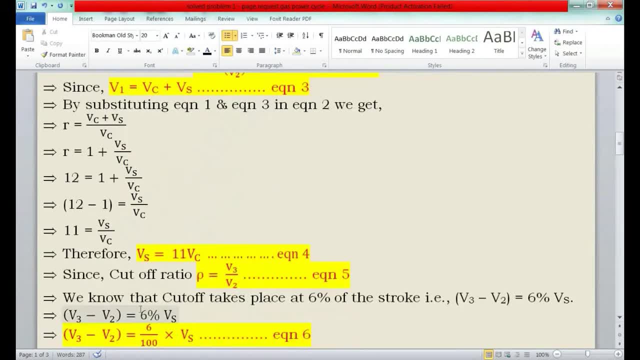 this clears this Vc to the LHS. So we get: Vs is equal to 11 times Vc, Or 11 Vc. Consider this one as equation 4, okay, So next is we will see cutoff ratio, Cutoff. 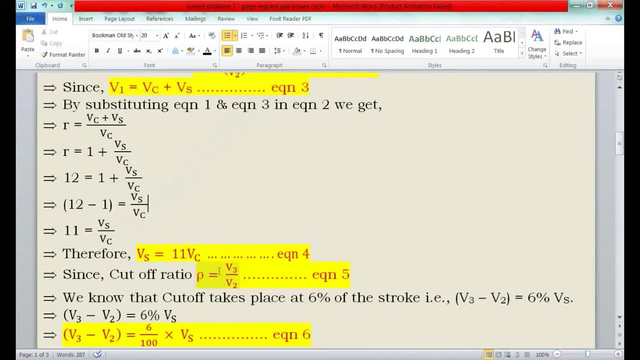 ratio is nothing but rho is equal to. I mean the formula for cutoff ratio is: rho is equal to V3 by V2.. That is volume at state 3 divided by volume at state 2, okay, So consider this one as equation. 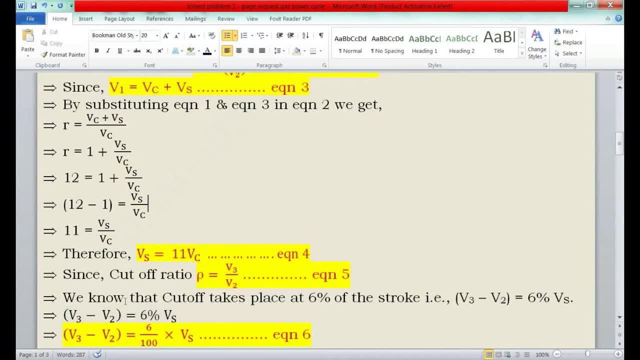 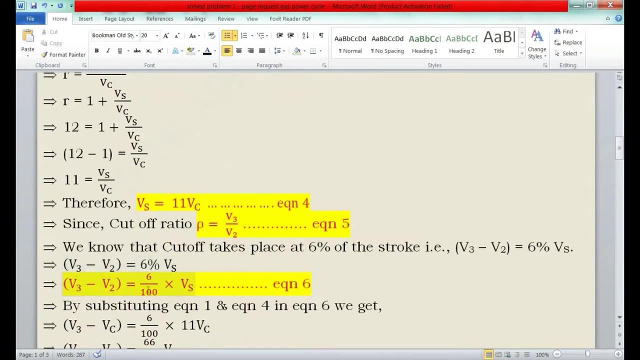 5,. okay, Already, we have a condition that cutoff takes place at 6 percent of the stroke. That is, V3 minus V2 is equal to 6 percent of Vs. okay, So this 6 percent is nothing but 6 by 100. Therefore, V3 minus V2 will be equal to 6 by. 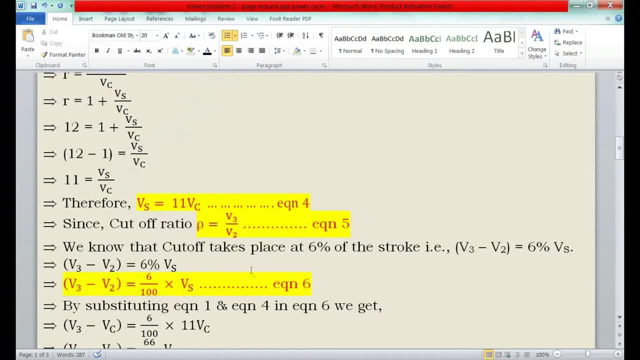 100 into Vs. Consider this one as equation 6.. Now substitute equation 1 and equation 4 in equation 6.. So we are going to substitute equation 1 and equation 4 in this equation 6.. What is equation? 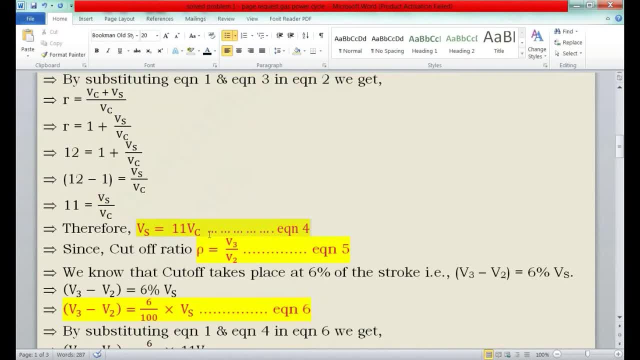 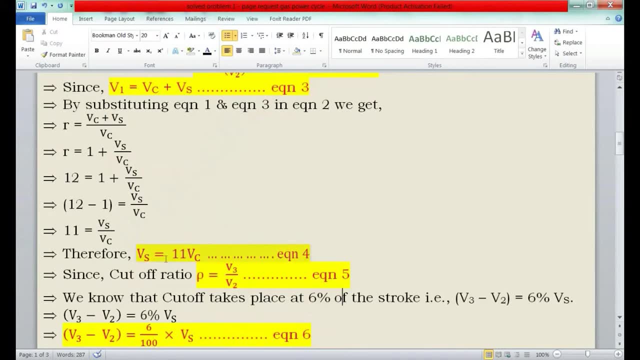 1?. Equation 1 is nothing but V2 is equal to Vc. okay, So this V2 will be replaced by Vc. And equation 4 is nothing but Vs is equal to 11 times Vc. So this Vs will be replaced by 11 times. 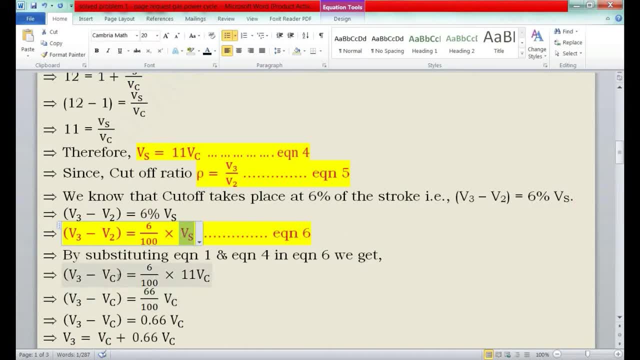 Vc, That is 11 Vc. Therefore, this equation will be modified as: V3 minus Vc is equal to 6 by 100 into 11 times Vc. okay, Or 11 Vc, okay. Now multiply this 11 into 6. We get 66. Therefore, 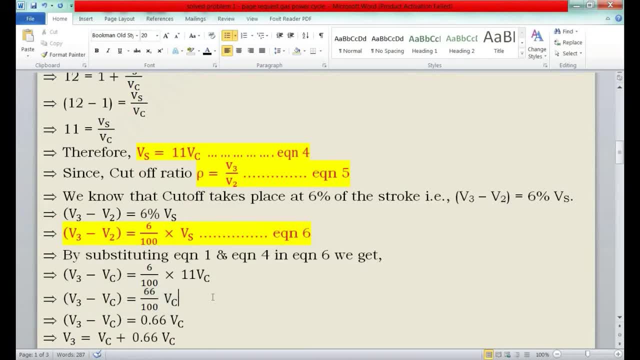 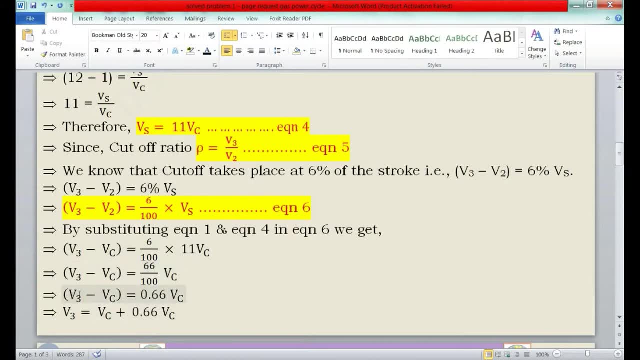 V3 minus Vc is equal to 66 by 100 into Vc. Okay, 66 by 100 is 0.66.. Therefore, V3 minus Vc is equal to 0.66 Vc. okay, Now move this Vc to. 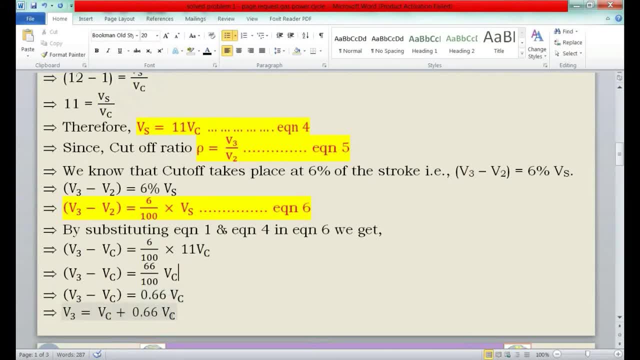 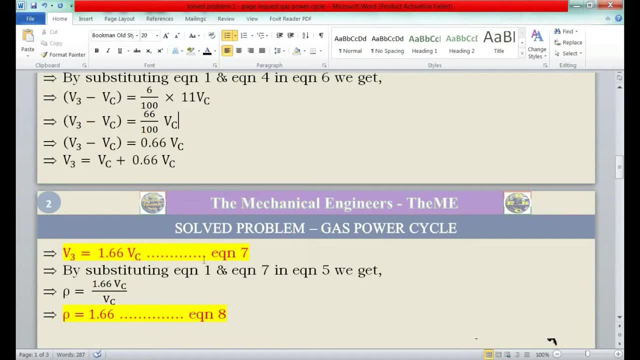 the RHS, We get: V3 is equal to Vc plus 0.66 Vc. Therefore, we will get: V3 is equal to 1.66 Vc. Consider this one as equation 7,. okay, Now substitute equation 1 and equation 7 in equation. 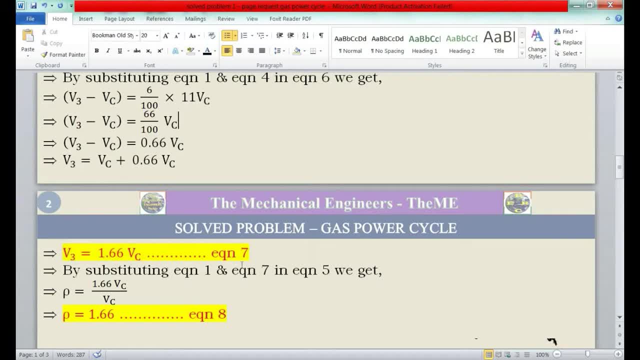 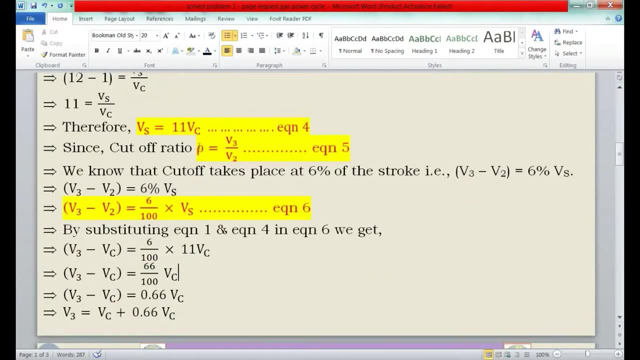 5. Equation 1 is nothing but Vc is equal to V2.. Equation 7 is nothing but V3 equal to 1.66 into Vc. So equation 5 is nothing but rho is equal to V3 by V2.. So 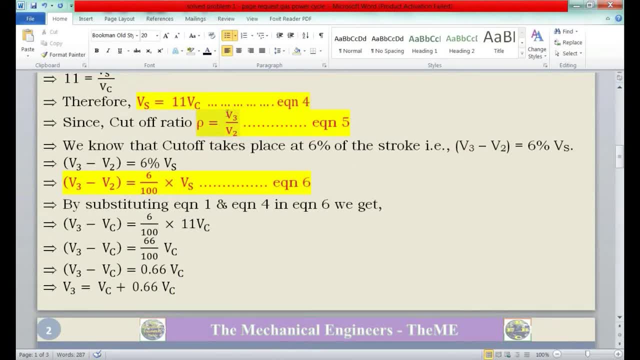 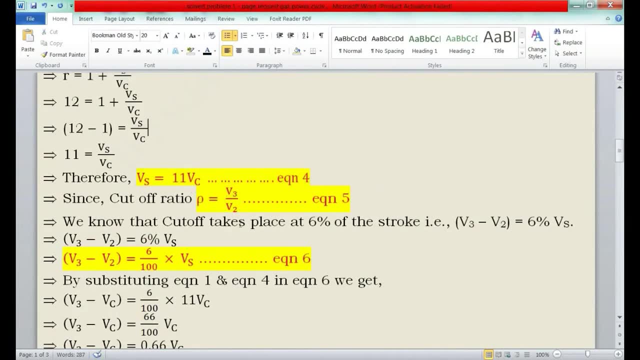 by substituting equation 7, this V3 will be replaced by 1.66 Vc- okay, 1.66 Vc. And by substituting equation 1, this V2 will be replaced by Vc. Therefore, this equation 5 will be modified. 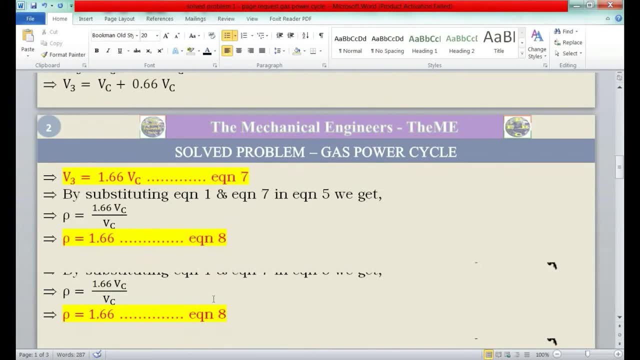 as this equation 5 will be modified as rho is equal to 1.66 Vc. So by substituting equation 5, rho is equal to 1.66 Vc by Vc. Therefore this Vc Vc get cancelled, We get rho is equal to 1.66. 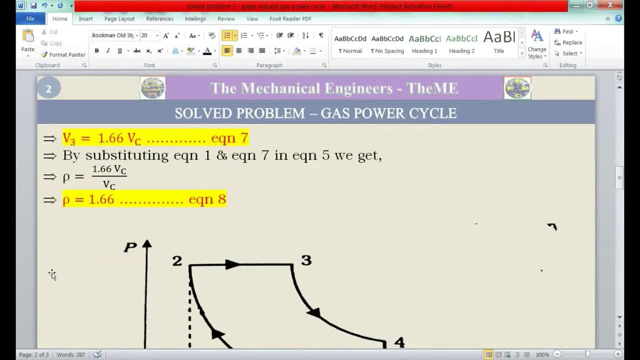 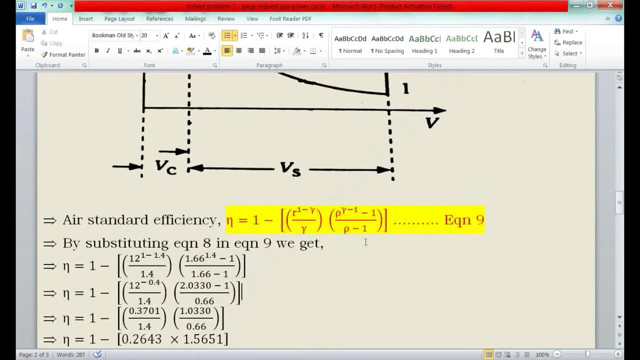 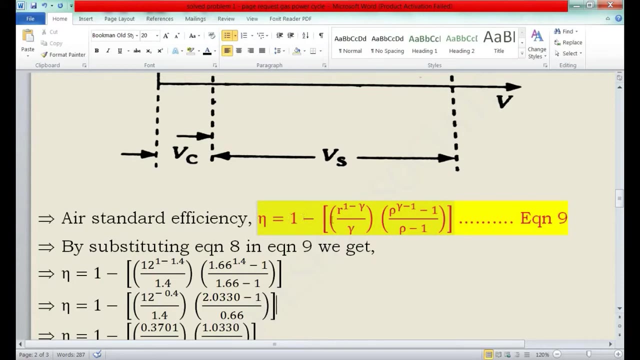 Consider this one as equation 8.. Next is air standard efficiency, And the formula for air standard efficiency of a diesel cycle is one sec. yeah, And the formula for air standard efficiency of a diesel cycle is Nita is equal to 1 minus R, to the power of 1 minus gamma divided by gamma. 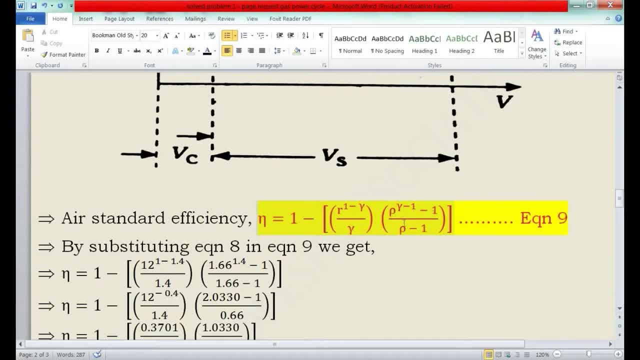 into rho to the power of gamma minus 1.. Minus 1 divided by rho minus 1,. okay, So here, Nita is air standard efficiency, or is compression ratio, which is 12.. And gamma is adiabatic constant And the universal value is 1.4. 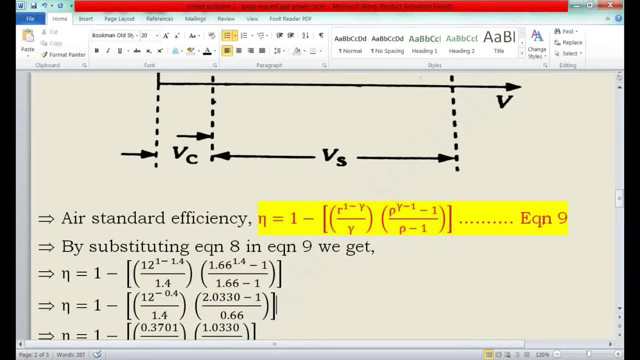 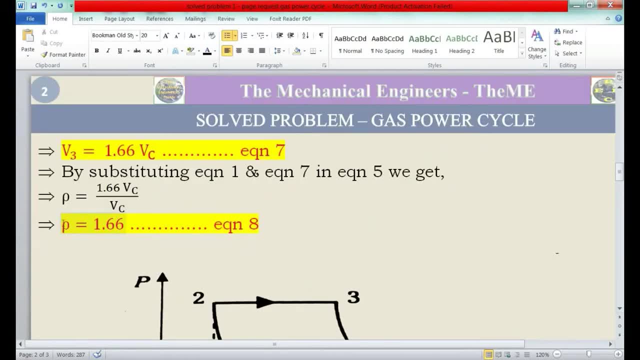 And the rho is cutoff ratio. okay, So consider this one as equation 9.. Now substitute equation 8 in equation 9.. What is equation 8? Equation 8 is nothing but rho value, which is 1.66.. So 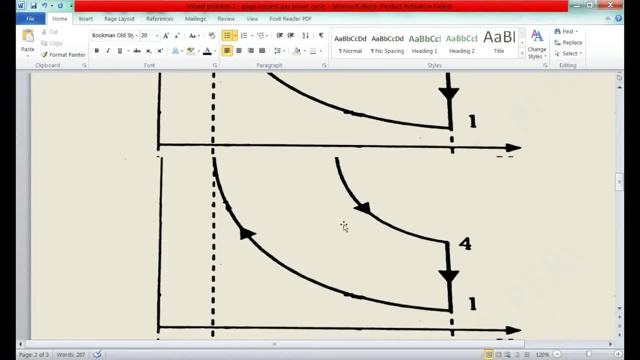 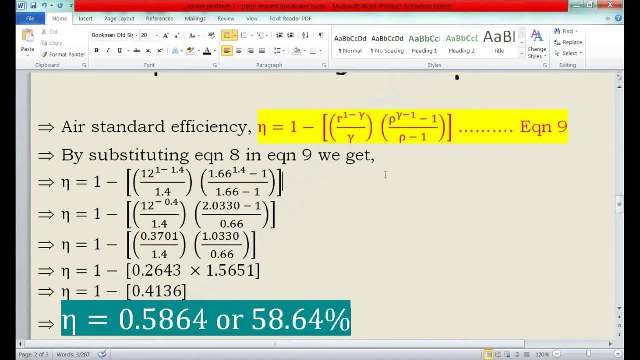 substitute this equation 8 in equation 9.. By substituting equation 8 in equation 9, this rho value will be replaced by 1.66.. So Nita is equal to 1 minus 12 to the power of 1 minus 1.4, divided by 1.4 into 1.66 to the power of 1.4. 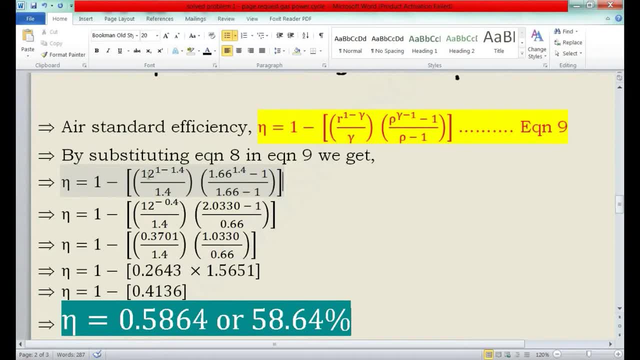 minus 1, divided by 1.66 minus 1.. So here, 12 to the power of 1 minus 1.4 is 12 to the power of minus 0.4.. And 1.66 to the power of 1.4 is 2.033.. 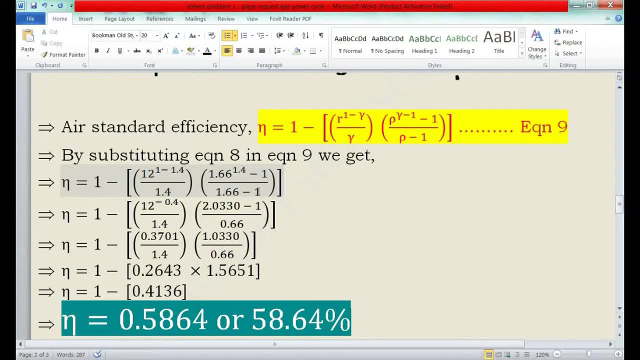 Okay, And 1.66 minus 1 is 0.66.. Therefore, this equation will be modified as: Nita is equal to 1 minus 12, to the power of minus 0.4 divided by 1.4, into 2.0330 minus 1 divided by 0.66.. Okay. 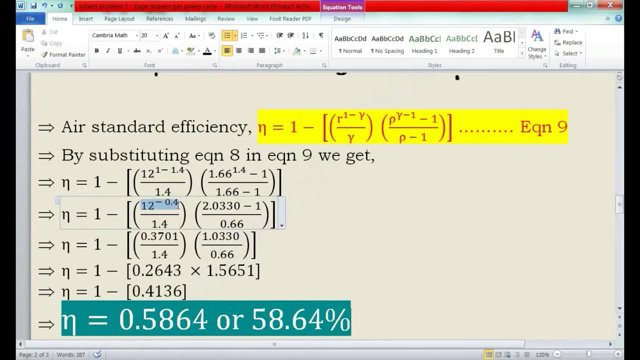 So the 12 to the power of minus 0.4 is 0.3701.. Okay, 12 to the power of minus 0.4 is 0.3701.. Okay, And this 2 point, sorry, and this 2 point, excuse me: 2.0330 minus 1 is 1.0330.. Okay. 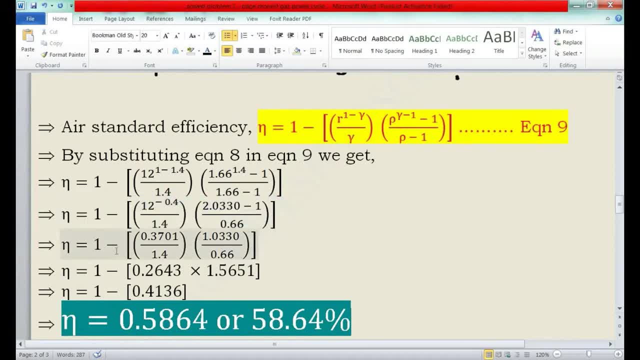 So this equation will be modified as Nita is equal to 1 minus 0.3701 divided by 1.4, into 1.0330 divided by 0.66.. So 0.3701 divided by 1.4.. Okay, So Nita is equal to 1 minus 0.3701 divided by 1.4. 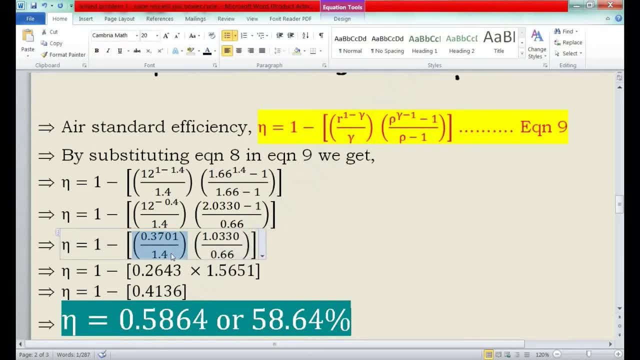 is 0.3701 divided by 1.4 is 0.2643.. And 1.0330 divided by 0.66 is 1.5651.. Therefore this equation will be modified as Nita is equal to 1 minus 0.2643 into 1.5651.. Okay. 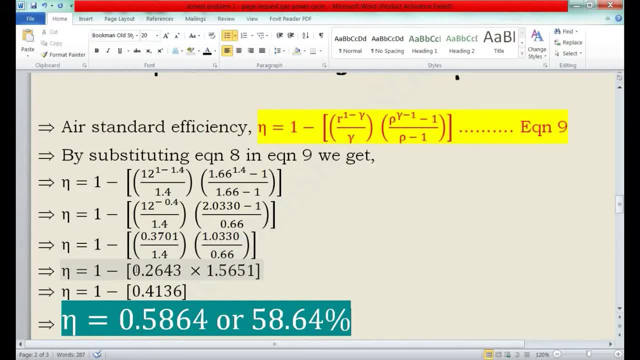 So 0.2643 into 1.5651 is 0.4136.. Therefore, this equation will be modified as Nita is equal to 1 minus 0.4136.. So 1 minus 0.4136 is Nita is.